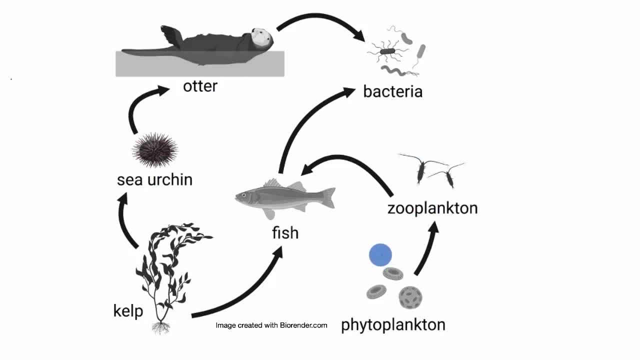 So this diagram right over here describes a food web, and a food web models how energy and matter moves in an ecosystem, And we're going to use this food web to answer some questions to make sure we understand food webs. So the first thing I'm going to ask you is: 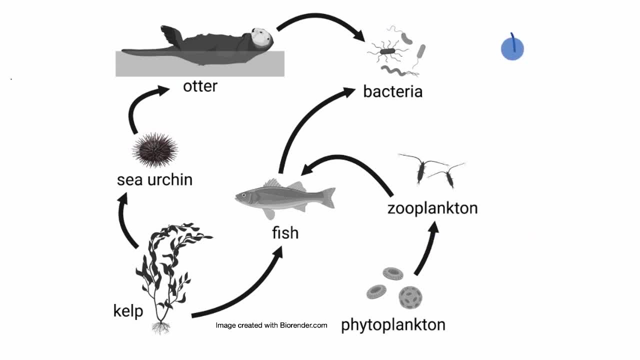 what are the producers in this food web? Pause this video and see if you can figure this out. All right, now let's work through this together. The producers are the ones that can take matter in the ecosystem, in the environment and energy from an outside source, usually the sun. 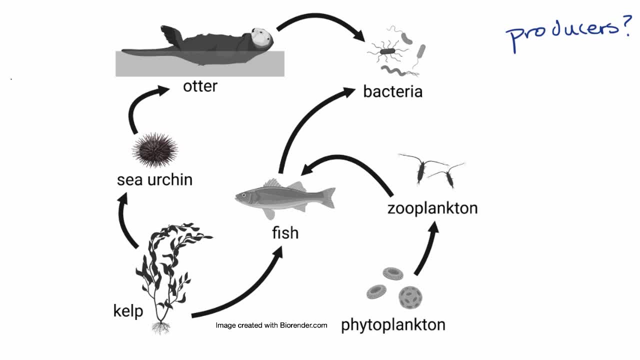 in order to construct themselves and also in order to store that energy. And when you look at a food web, producers are going to have arrows pointed away from them, So they're getting their energy and their matter from the environment and then other people are going to consume them. 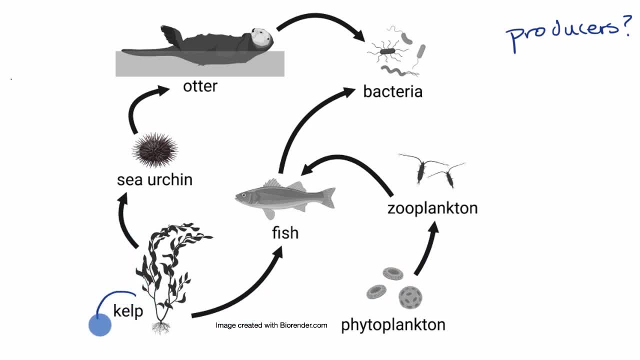 and we're going to talk about them in a little bit, But we can see here that the kelp is a. the kelp is a producer. This is an aquatic ecosystem that we're looking at, but the kelp is a producer. 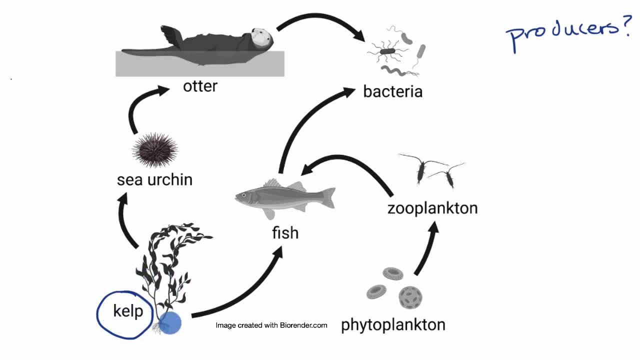 There's no arrows going into it, So it's using the sun and elements and atoms and molecules that it's finding in its environment in order to grow, And we can also see that's the case with the phytoplankton. It's also able to do photosynthesis, like the kelp. 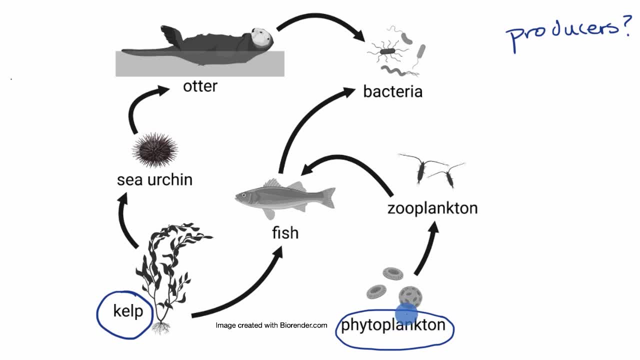 and capture that energy from the sun. Now the next question I have is: where are the decomposers? Pause the video and try to answer that one. All right now you might remember decomposers you can think about. that's where a lot of the energy and the matter. 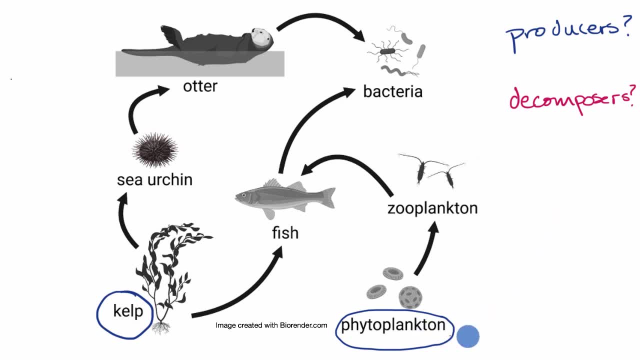 ends up to be decomposed and then recycled again and be reused again by the producers- And if you're looking at a food web, it's. these would be organisms where all of the arrows point to them, but you don't have any arrows coming from them. 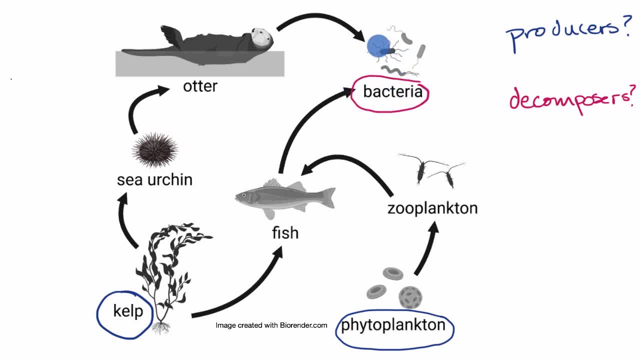 And over here it's clear that the bacteria- and there's many different species of bacteria or many different types of bacteria, but the bacteria here are the decomposers. Next, I am going to ask you about the primary, primary consumers.